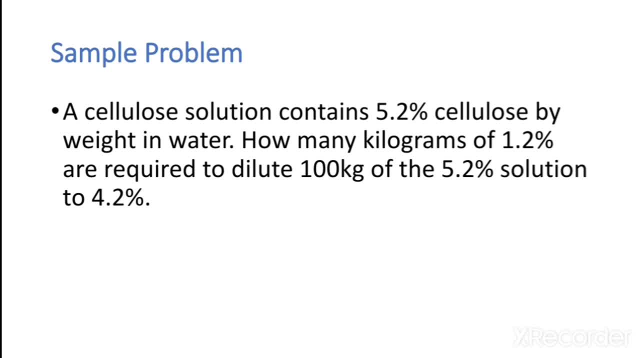 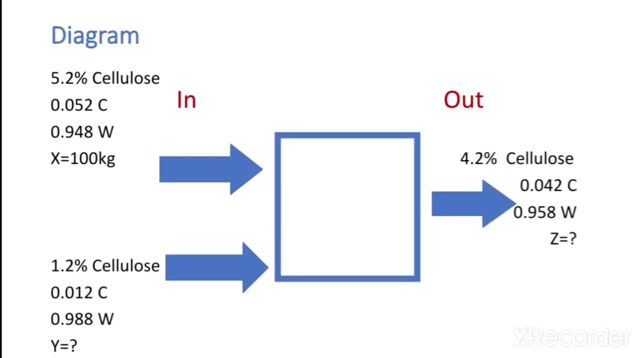 mass is 100 kg. we have to find the mass of second stream. gather all the information in a diagram so that you can easily solve this problem. so we have two stream coming in. i have drawn two arrow here. coming in to a box and one stream is coming out means we are getting only one product. so as we have only two components, 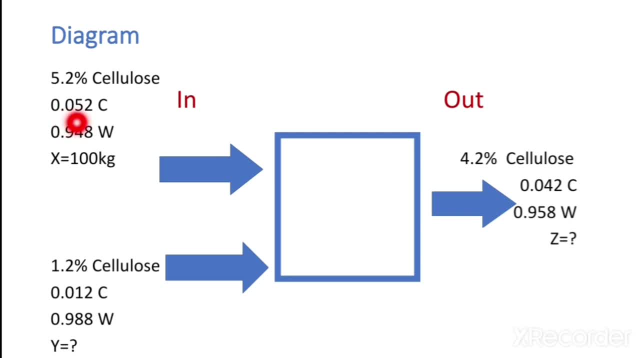 cellulose and water. so if 0.052 is fraction of cellulose then water fraction would be 0.948 and as we have been given 100 kg total flow rate, so i have written here. similarly, 1.2 percent concentration of cellulose was given for stream 2, so i have written fraction here for cellular it's. 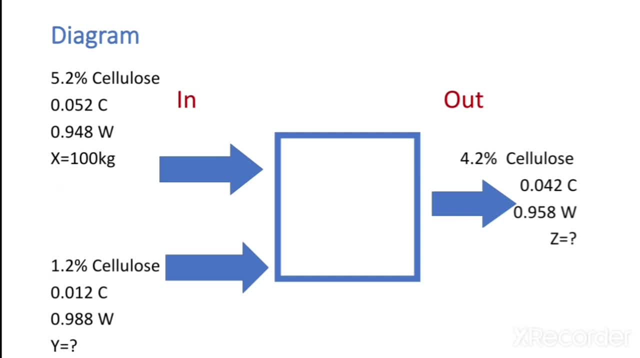 0.012 and fraction of water in stream 2 is 0.9. double it and we have to find the value. of y means the total flow or total mass of stream 2. and 4.2 percent is the concentration required for this stream and we also don't know the total stream of flow stream coming out of system. 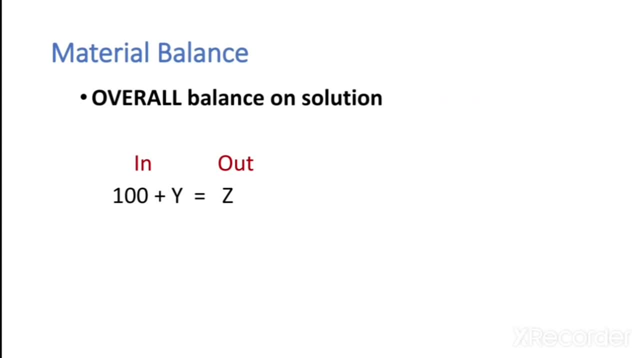 and you can also to be the solution to solve this problem with all equations, and we can also be the solution for this problem with all equations. so we have to find the solution to solve this problem. so here we have 2 possible solution. first, we apply overall balance on solution. what is overall balance? overall balance is: 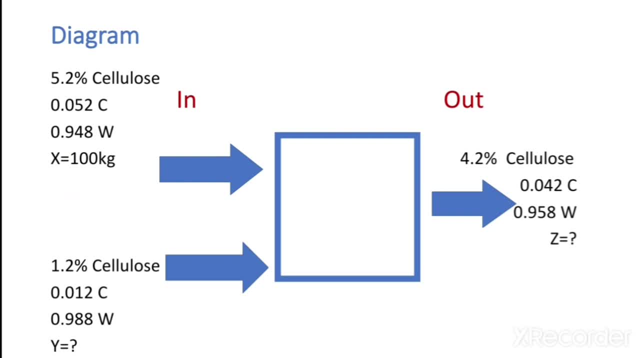 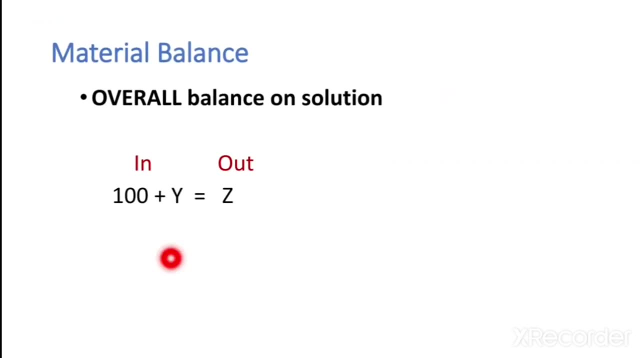 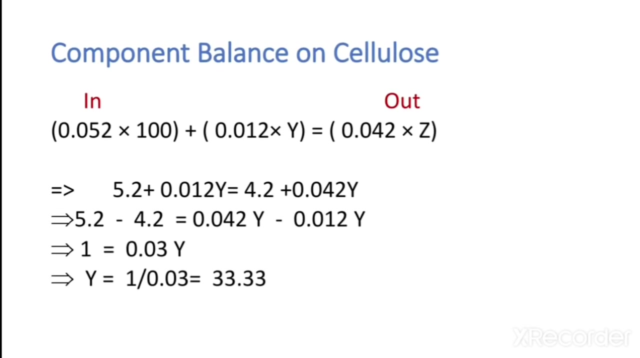 total flow of all streams means total flow coming in is, some of which is which is shown by Z, which is also unknown. so we can write this in equation here: 100 plus I is equal to Z. so when we apply component balance on cellulose, cellulose in stream 1 was 0.052 fraction multiplied by total flow. 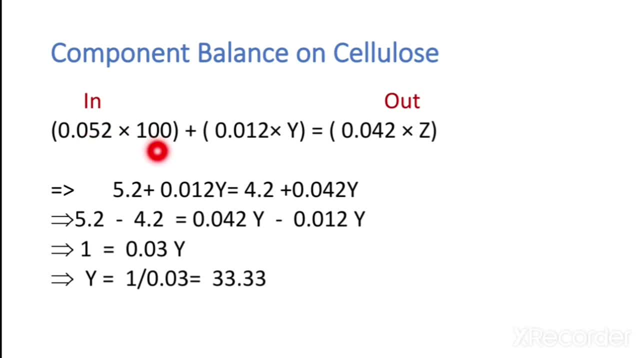 of stream 1, total flow was given, which is 100, and similarly cellulose in stream 2 was 0.012 fraction, or 1.2 percent of total flow. flow stream is Y, because we don't know the value, so we will add up the total incoming cellulose, which is: 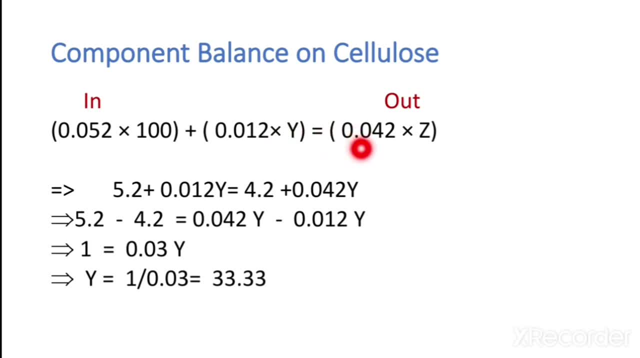 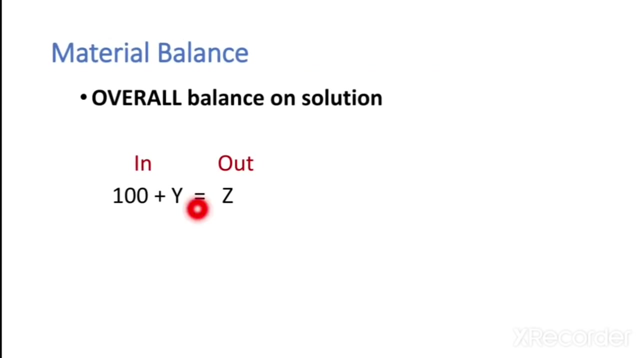 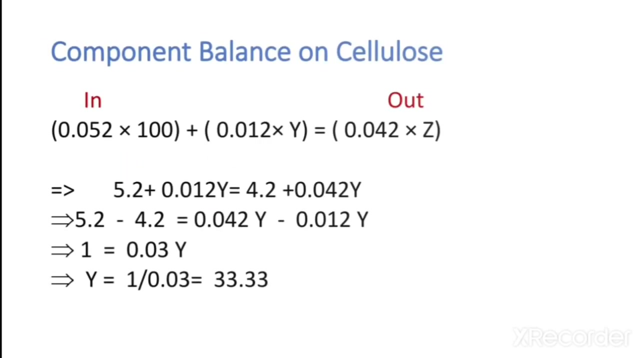 equal to total out coming cellulose, which is 0.042 fraction multiplied by total flow of stream. we have solved this and we get that Y is equal to 33.33. if we put this in very first equation here, then we can find that Z is equal to 1, 33.3. so 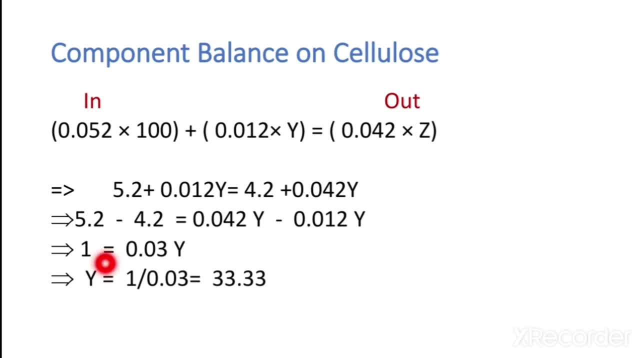 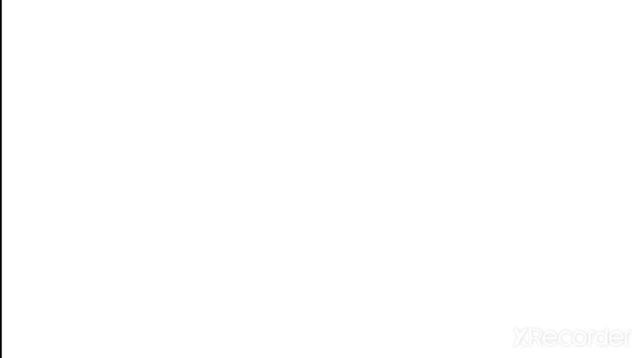 although we have find the unknown variable, which is Y, we can solve it. for alimentкт time, Zenin best expression is the paradigm Skip test and type tough question in CAT'srint Test. for second component, balance, we can apply balance on water and solve this equation to. 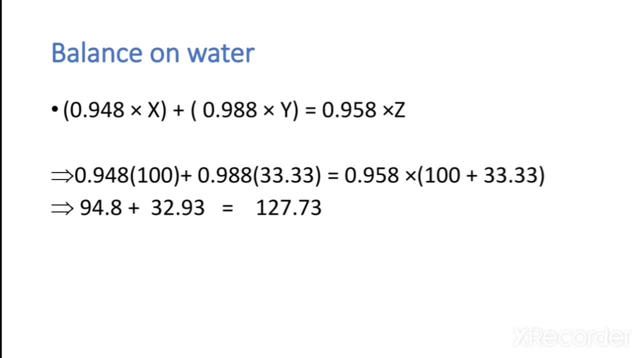 check whether we have find the exact value or any error has been happened. so when we apply water balance on system, we find here: total water coming in stream 1 can be calculated by multiplying fraction with total flow, and total flow of water coming from stream 2 is. 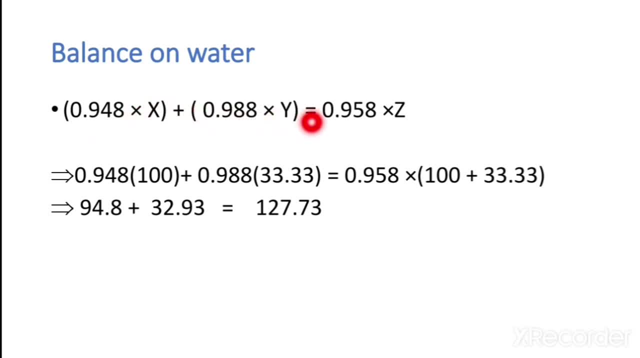 here. add up both stream, which is equal to total flow of water coming out of stream 3. so we put the known variable here: x is equal to 100, y is equal to 33.33, z is equal to 133.33. we can see here: left hand side and right hand sides are equal. 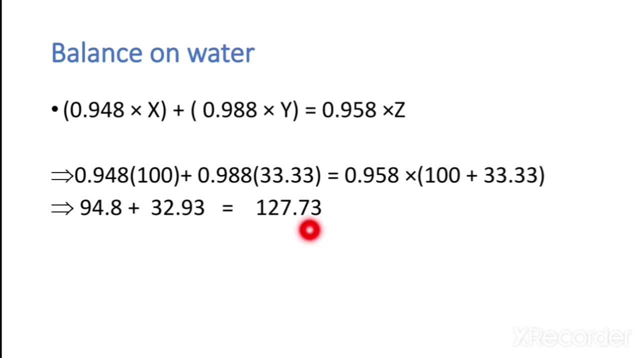 so we can see here left hand side and right hand sides are equal, which means we have find the correct values. if you have liked my video, please like, comment and subscribe. best of luck.